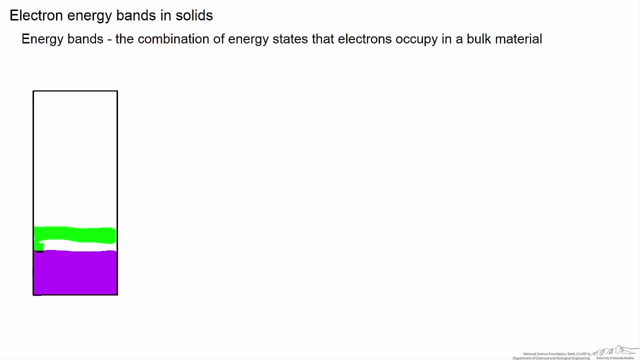 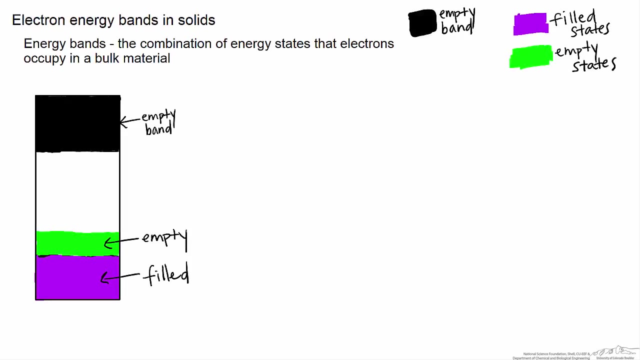 here in green. Electrons can easily move into these states and are thus available for electrical conduction in the material. There is also an energy band at higher energy in these materials, but that band is unused since there are empty states directly adjacent to the filled states. 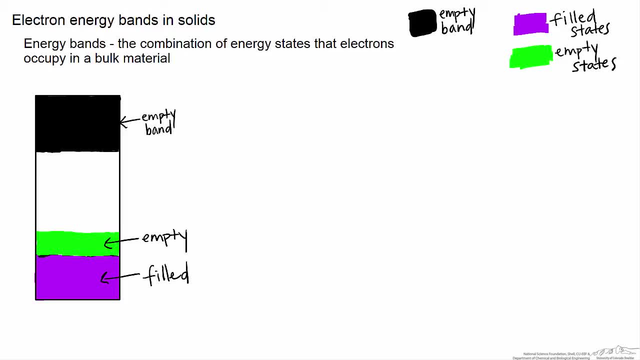 That empty band is shown here in black. The next type of material I will discuss is a different type of metals, Unlike copper, which has only one electron in its 4s orbital and is capable of accommodating two electrons in that orbital, thus the empty states in that electron band. metals such as magnesium. 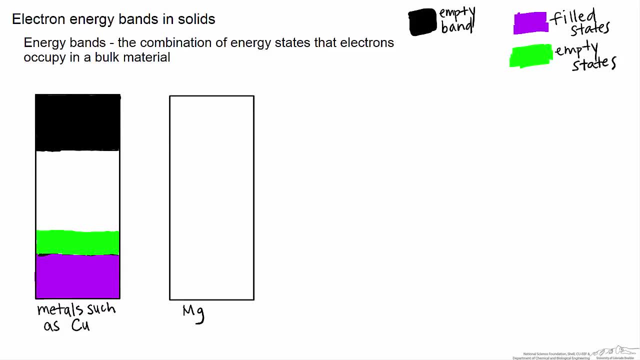 have a filled 3s orbital. However, there is an adjacent orbital, The 3p orbital, that can accommodate electrons. Though this orbital overlaps, it does take a little bit of energy to get electrons into it, and thus magnesium is a slightly less good conductor of electricity than copper. 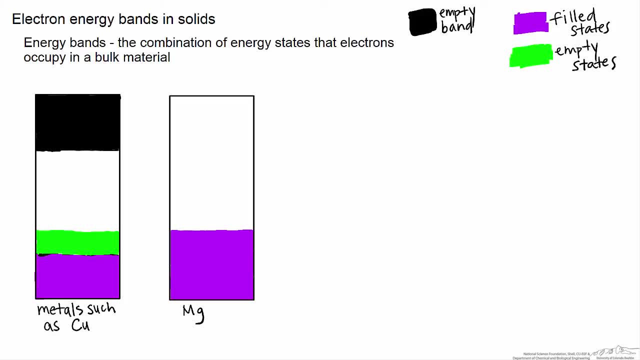 is Again, just to reiterate: unlike copper, magnesium doesn't have an unfilled state. It has an adjacent empty band where the band in terms of energy is adjacent to the filled states. Thus it is very easy for electrons to enter that band and be available for conduction. 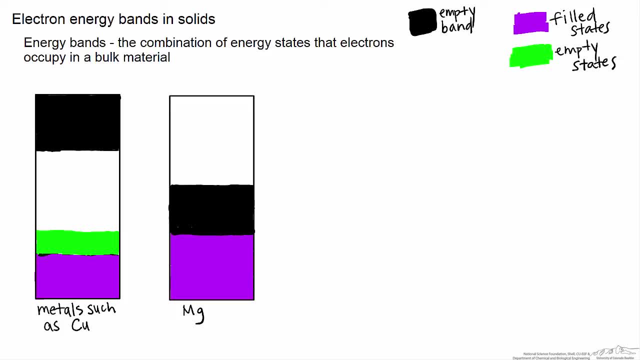 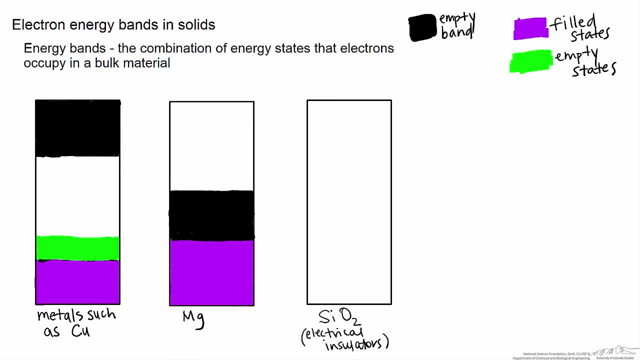 The empty band is shown here in black. The next type of material I will discuss is electrical insulators like silicon dioxide. These materials, often ceramics, have filled energy states, just like the other two. However, their empty band is significantly farther away in terms of energy. This energy differential. 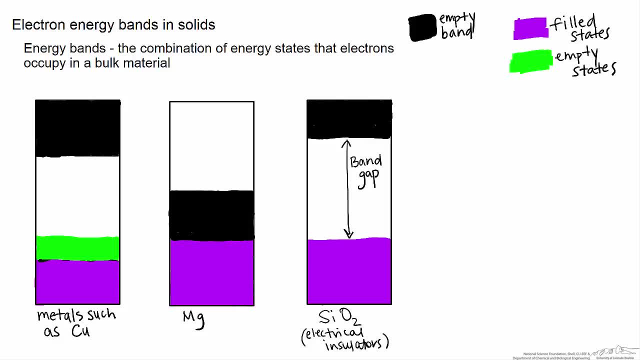 called the band gap For insulators. this band gap has an energy that is usually much greater than two electron volts. The final type of material is semiconductors. These materials, such as silicon, have a similar band structure to insulators, where, again, 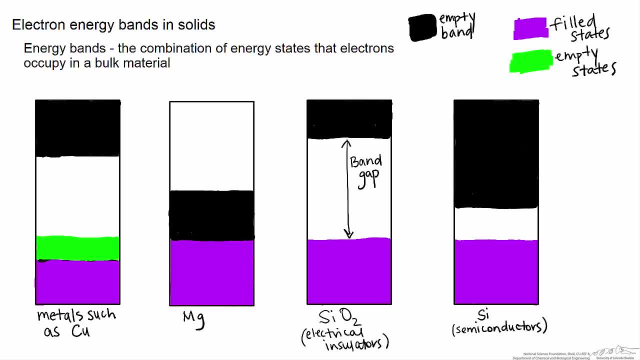 they have filled states and an unfilled energy band. that is slightly different in energy. However, unlike the insulating materials, the band gap here is very small in terms of energy, where it has about two electron volts or less difference between the top of the filled states and the empty band.